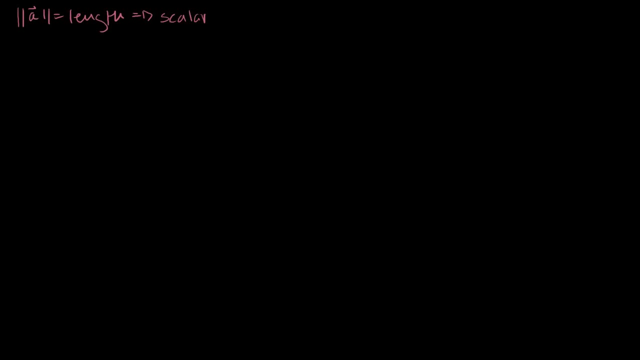 In this video I want to attempt to define the notion of an angle between vectors. As you can see, we're building up this mathematics of vectors from the ground up And we can't just say, oh, I know what an angle is, because 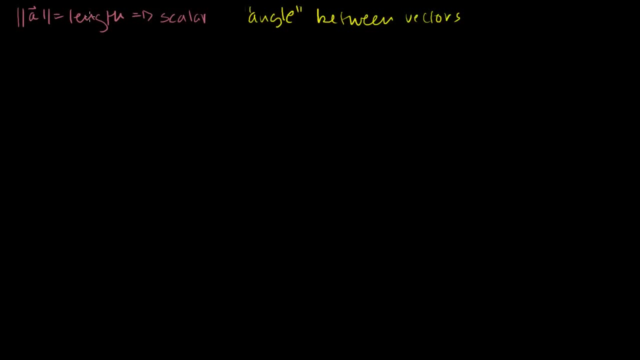 everything we know about angles and even lengths. it just applies to what we associate with two- or three-dimensional space. But the whole study of linear algebra is subtracting these ideas into multi-dimensional space, And I haven't even defined what dimension is yet, but I 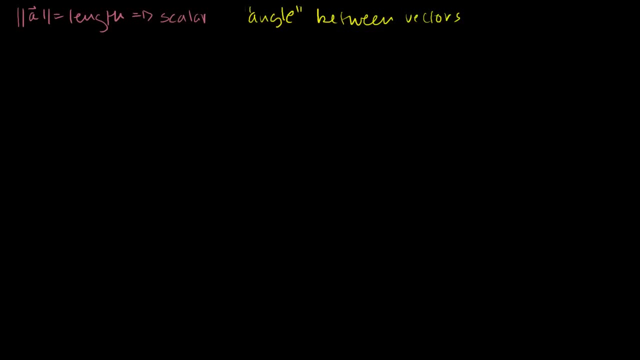 think you understand that idea to some degree already when people talk about one or two or three dimensions. So let's say that I have some vector. Let's say I have two vectors, Vectors a and b. They're non-zero And they're members of r. 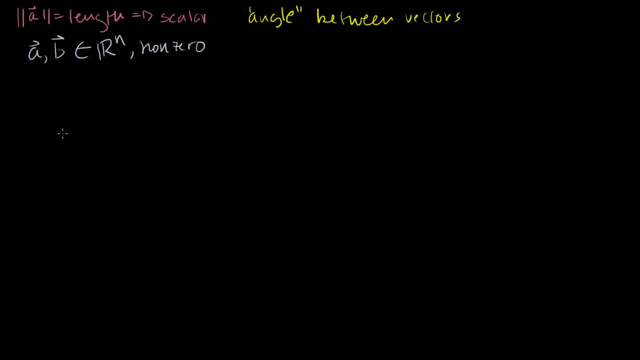 And they're non-zero. And they're members of r And they're members of r And they're non-zero. And I don't have a notion of the angle between them yet, But let me just draw them out. Let me just draw them as if I could draw. 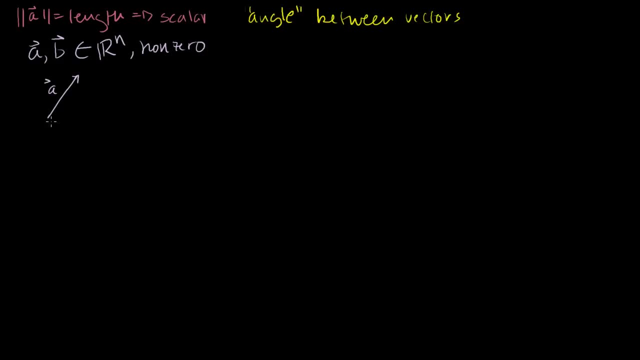 them in two dimensions. So that would be vector a right there, Maybe that's vector b right there, And then this vector right there would be the vector a minus b, And you can verify that just the way we've learned to add and subtract vectors. 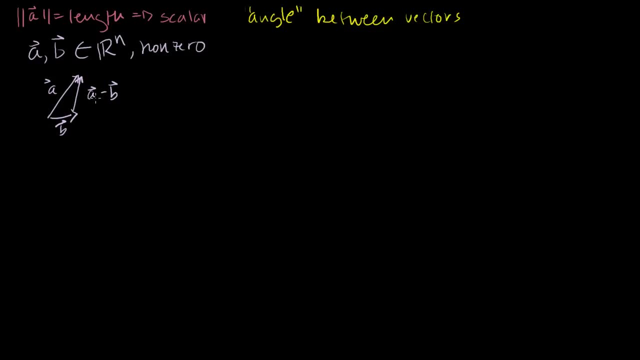 Or this is heads to tails, So b plus a minus b is of course going to be vector a, And that all just works out there. To help us define this notion of angle, let me construct another triangle that's going to look a lot like this one. 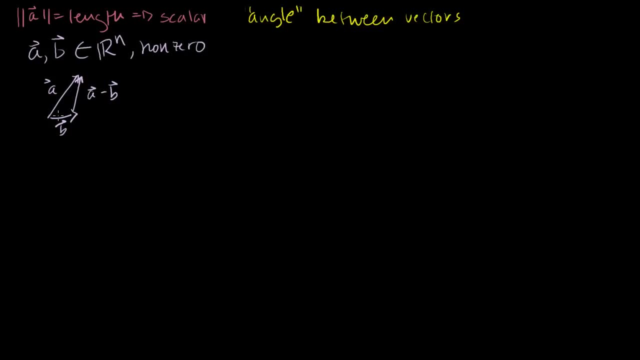 But remember, I'm just doing this for our simple minds, to imagine it in two dimensions. But these aren't necessarily two-dimensional beasts. These each could have 100 components. But let me make another triangle. Let me make another triangle that looks something similar. 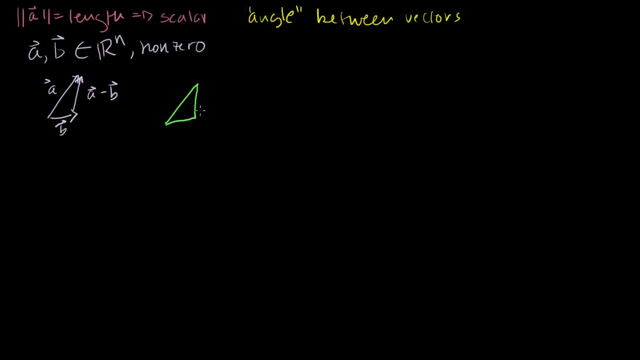 Say, it looks like that, And I'm going to define the sides of the triangles to be the lengths of each of these vectors. Remember the lengths of each of these vectors. I don't care how many components they are, They're just going to be your numbers. 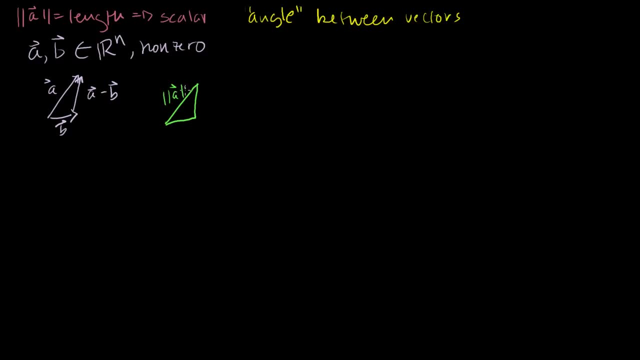 So the length of this side right here is just going to be the length of a. The length of this side right here is just going to be the length of vector a minus vector b, And the length of this side right here is going to be the 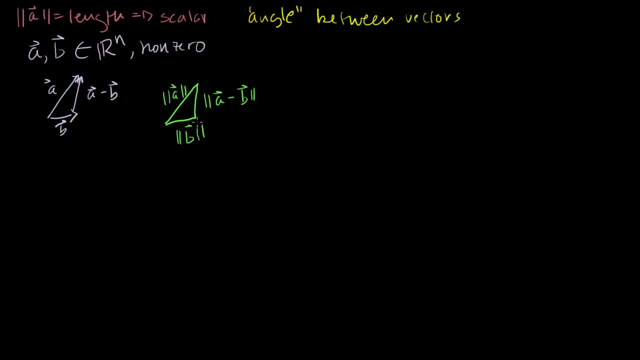 length of vector b. Now, the first thing we want to make sure is that we can always construct a triangle like that, And so under what circumstances could we not construct a triangle like this? Well, we wouldn't be able to construct a triangle like this. 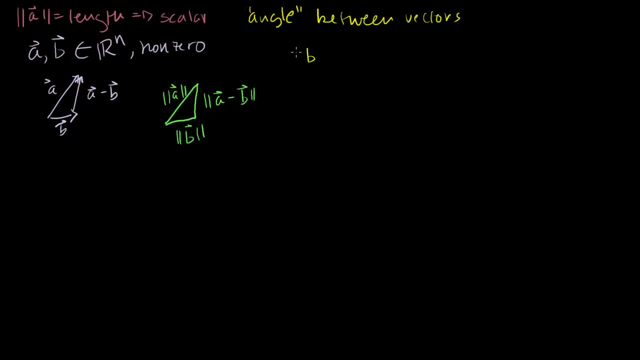 if this side, if b, if the magnitude. So let me write this down. That's kind of a subtle point, but I want to make this very clear In order to define an angle. I want to be comfortable that I can always make this connect. 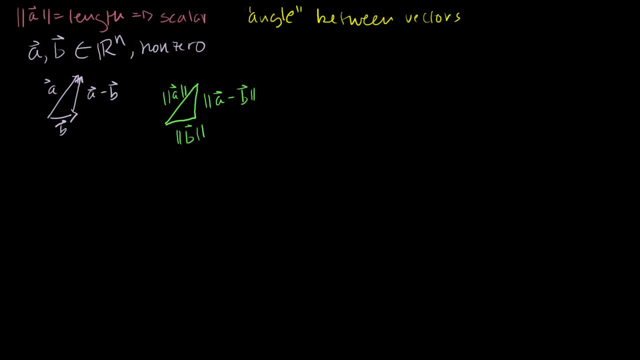 And I need to make sure that. let me write reasons why I couldn't, Reasons why I couldn't make this construction. Well, what if the magnitude of b was greater than, or the length of vector b was greater than, the length of vector a? 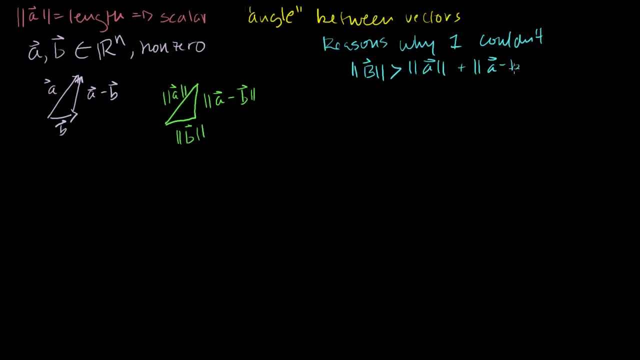 plus the length of vector a minus b In two dimensions. I could never draw a triangle like that then, Because you would have this length plus this length would be shorter than this thing right here, and so you could never construct it And I could do it with all the sides. 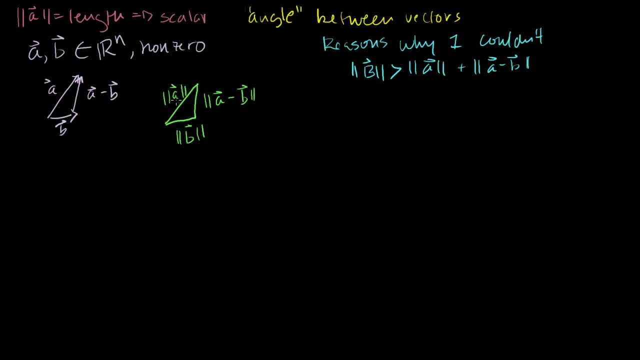 What if this length was larger than one of these two sides? Or what if that length was larger than one of those two sides? I could just never draw a two-dimensional triangle that way. So what I'm going to do is I'm going to use the vector. 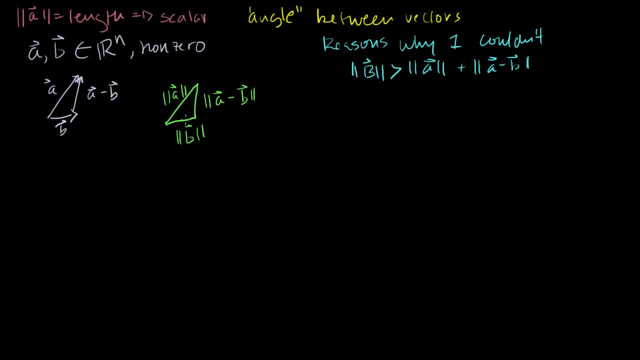 triangle inequality, to prove that each of these sides is less than or equal to the sum of the other sides. And I could do the same thing. Let me make the point clear. I could show that if a, for whatever reason, was greater than the other sides plus b, then I wouldn't be able to. 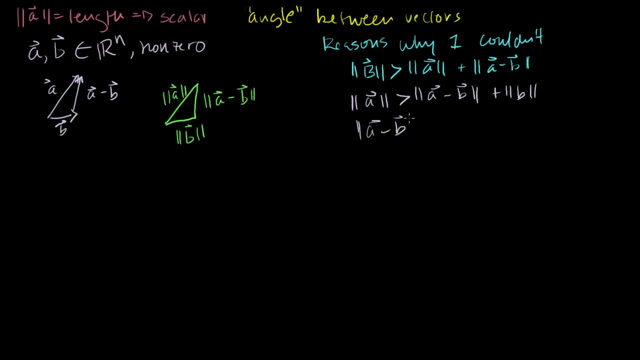 create a triangle. And the last one, of course, is if a minus b, for whatever reason, was greater than the other two sides, I just wouldn't be able to draw a triangle than a plus b. So I need to show that for any vectors that are any real. 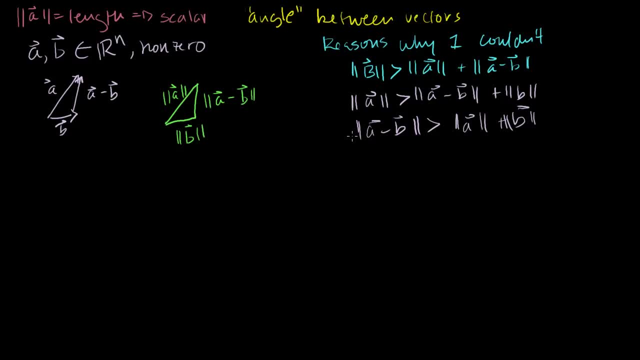 vectors, non-zero real vectors that are members of Rn, that's that none of these can ever happen. I need to prove that none of those can happen. So what does the triangle inequality tell us? The triangle inequality tells us that if I have the sum of 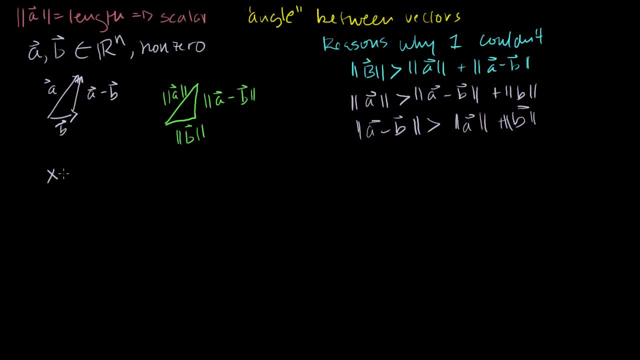 two vectors. if I take the length of the sum of two vectors, that that is always going to be less than- and these are non-zero vectors- is always going to be less than or equal to the sum of each of their individual lengths. 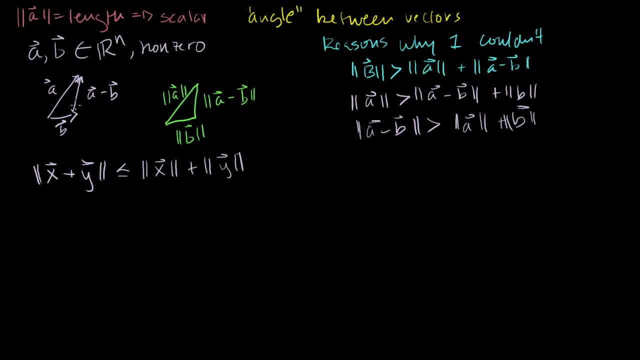 The sum of each of their individual lengths. So let's see if we can apply that to this triangle right here. So what is the magnitude, the length of a, The length of a? well, I can rewrite vector a. What is vector a equal to? 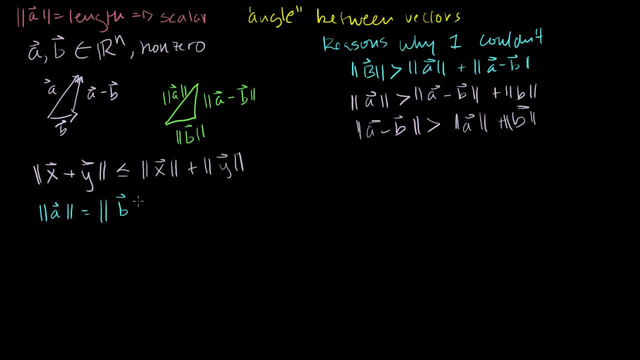 Vector a is equal to vector b plus vector a minus b, right? This is just. I mean, I'm just rewriting the vector here. I'm just rewriting a here as a sum of the other two vectors. Nothing fancy there. I haven't used the triangle inequality or anything. 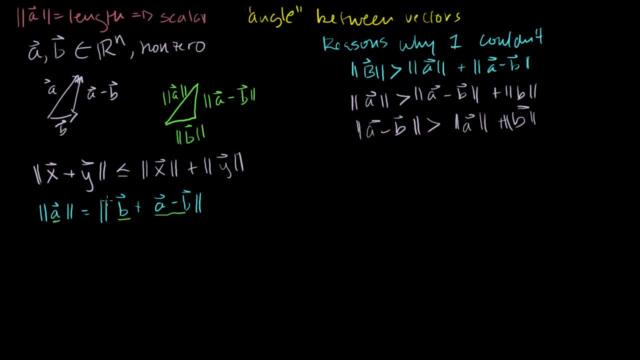 I've just used my definition of vector addition. But here now, if I put little parentheses, here now I can apply the triangle inequality and say: well, you know what This is going to be by the triangle inequality which we proved, it's going to be less than or equal to the lengths. 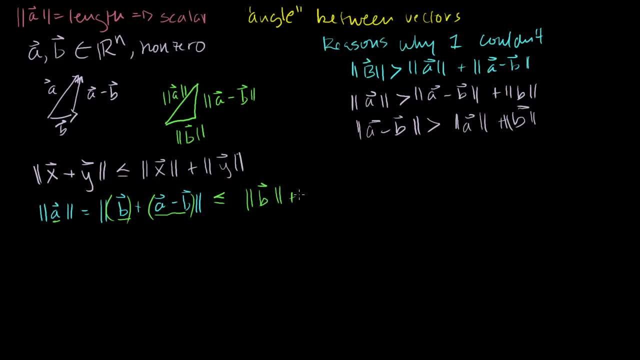 of each of these vectors, Vector b plus the length of vector a minus b. So we know that a is a. the length of a is less than the sum of that one and that one, So we don't have to worry about this being our problem. 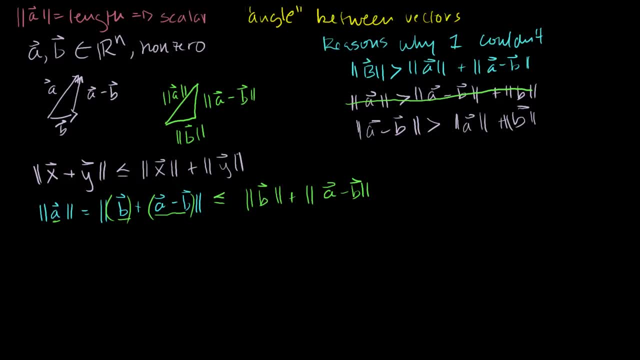 We know that that is not true. Now let's look at b. So is there any way that I can rewrite b as a sum of two other vectors? Well, sure, I can write it as a sum of a plus. let me put it this way: 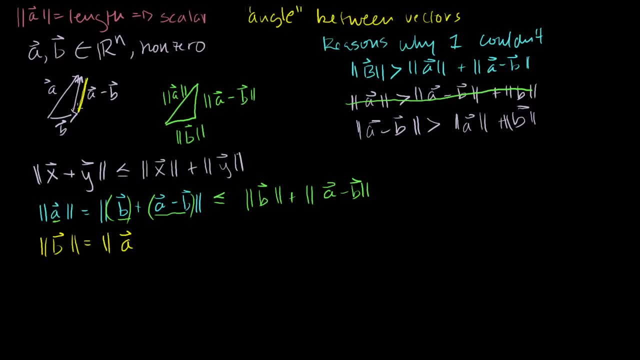 If that vector right there is a minus b, the same vector in the reverse direction is going to be the vector b minus a. So a plus the vector b minus a. that's the same thing as b And you can see it right here. 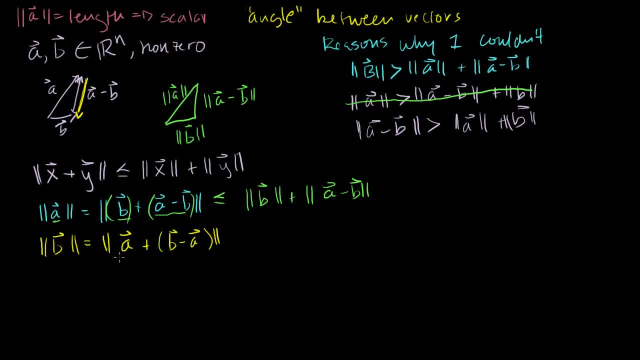 The a's would cancel out and you're just left with a- b. there Now, by the triangle inequality, we know that this is less than or equal to the length of vector a plus the length of vector b minus a. Now you're saying: hey, Sal, you're dealing with b minus a. 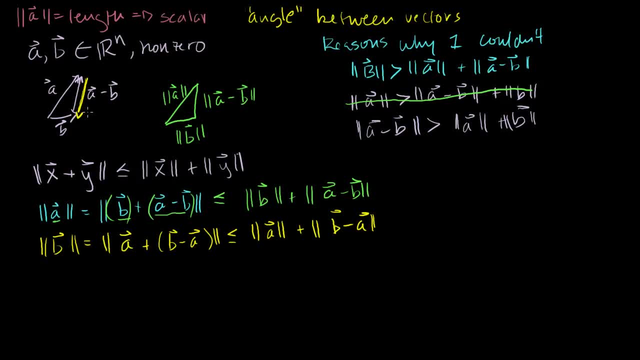 This is the length of a minus b And I could leave this for you to prove it based on our definition of vector lengths. But the length of b minus a is equal to minus 1 times a minus b And I'll leave it to you to say that. look these lengths. 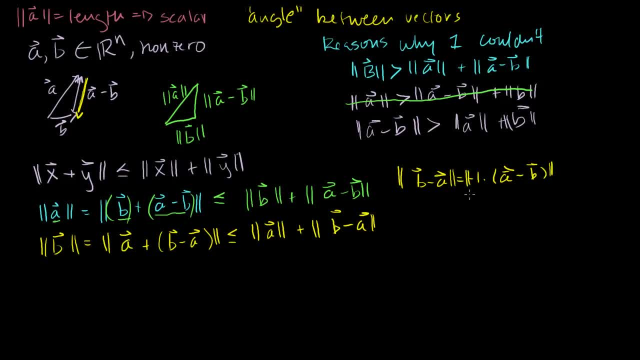 are equal Because essentially- well, I could leave that, but I think you can take that, based on just the visual depiction of them, that they're the exact same vectors just in different directions. And I have to be careful with length because it's not just. 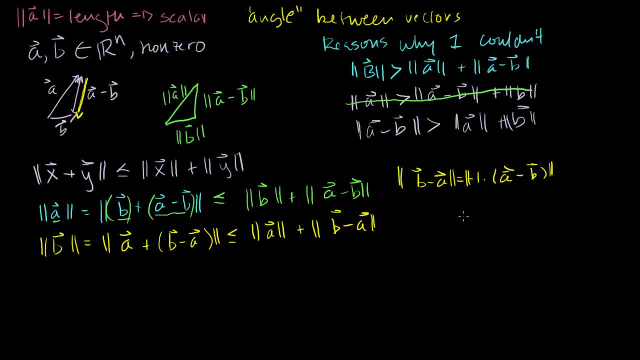 in two dimensions. But I think you get the idea- and I think I'll leave that for you to prove- that these lengths are the same thing. So we know that b is less than the length of those two things, So we don't have to worry about that one, right there. 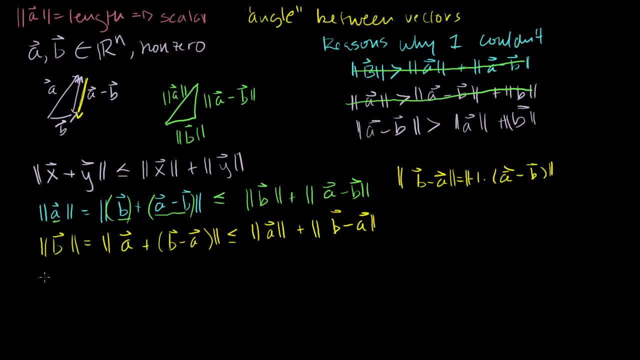 Finally, a minus b. can we write that the magnitude or the length of vector a minus b? Well, I can write that as vector a plus vector minus b. If we just put a minus b right there and go in the other directions, we could say minus b. 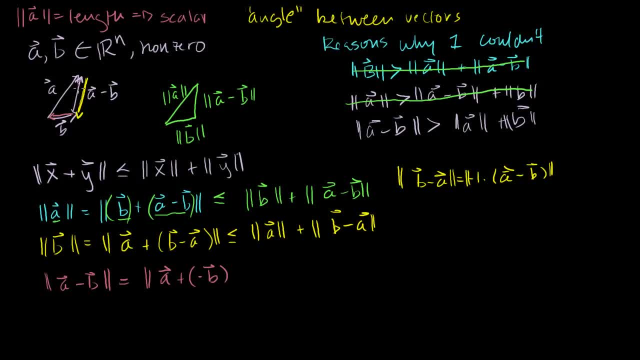 Which would be in that direction. Plus a would give us our vector a minus b, And that's obvious. Actually, I don't even have to go there, That's obvious from this. I just kind of put the negative in the parentheses. 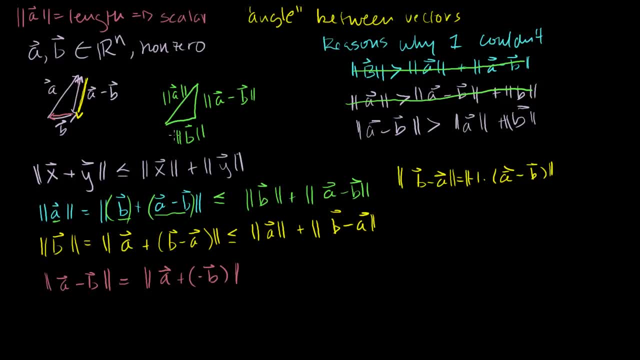 Well, the triangle, inequality- and this might seem a little mundane to you, but it really shows us that we can always define a regular planar triangle based on these vectors in this way- Tells us: this is less than or equal to the length of our 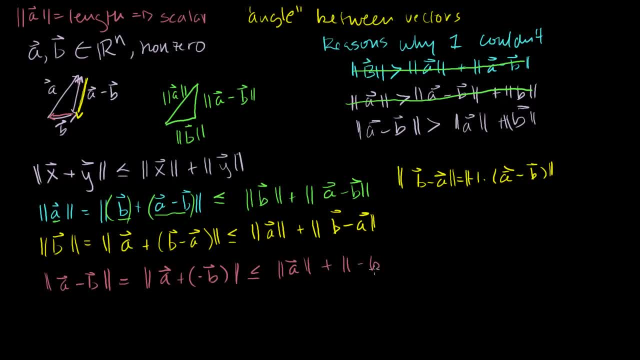 vector a plus the length of minus b, And I just said, and you could prove it to yourself, that this is the same thing as the length of b. So we just saw that this is definitely less than those two. this is definitely less than those two and that is. 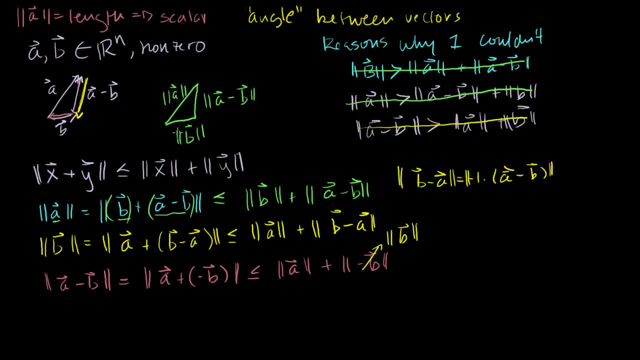 definitely less than those two. So we don't have none of the reasons that would keep us from constructing a triangle are valid. So we can always construct a triangle in this way. from any arbitrary non-zero vectors in Rn, We can always construct this. 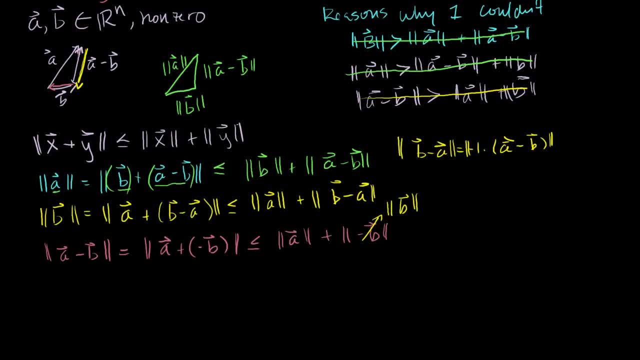 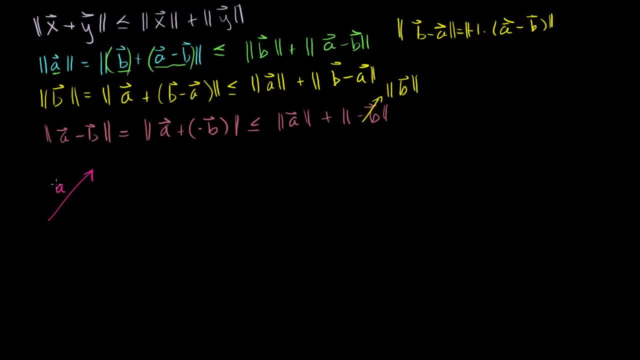 Now to define an angle, Let me Let me redraw it down here. Let me redraw the vectors, maybe a little bit bigger. That's vector a. I'll draw it slightly. This is vector b, And then let me just draw it this way. 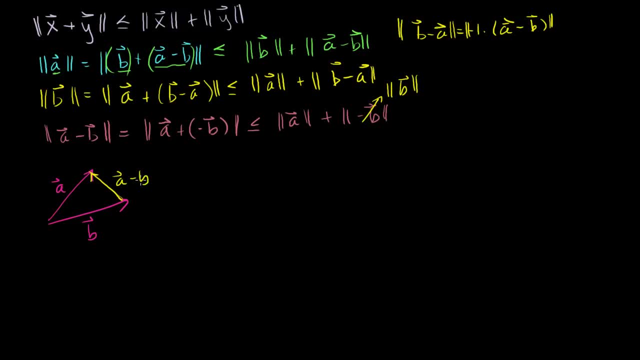 This is the vector right there, That's the vector a minus b, And we said we're going to define a corresponding regular run-of-the-mill vanilla triangle whose lengths are defined by the lengths of the vectors, by the vector lengths. So this is the length of b. 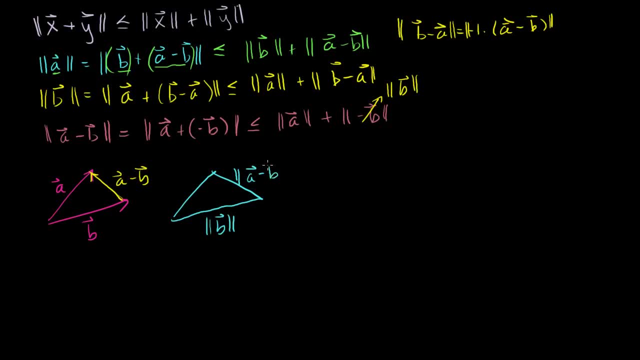 That side, This is the length of a minus b, And then this is the length of a. Now, now that I know that I can always construct a triangle like this, I can attempt to define- actually I will define my definition- of an angle between two vectors. 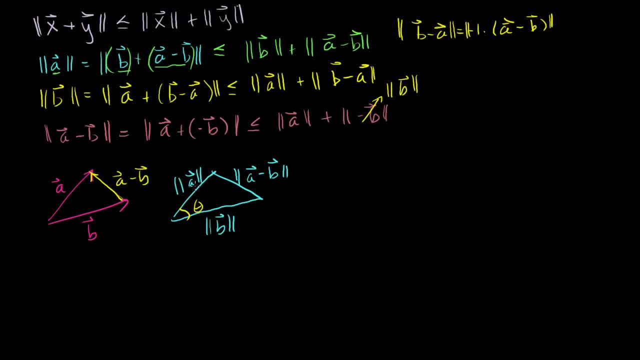 So we know what an angle means in this context. This is just a regular run-of-the-mill geometric triangle. Now my definition of an angle between two vectors. We can just cut and draw in like this: between two vectors. I'm going to say so, this is what I'm. 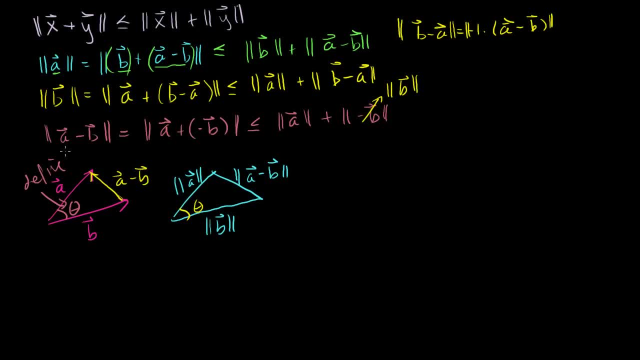 trying to define because these can have arbitrary number of components so it's hard to visualize. But I'm going to define this angle as the corresponding angle in a regular run-of-the-mill triangle where the sides of the run-of-the-mill triangle are: 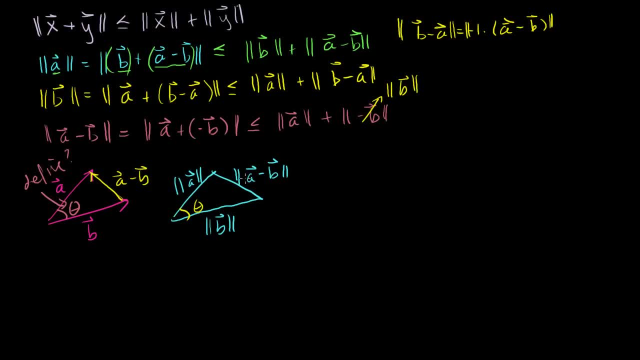 the two vectors and then the opposite side is the subtraction is the length of the difference between the two vectors. This is just the definition. I'm just saying that these two things, I'm defining this, the angle between two vectors in Rn that could have an arbitrary. 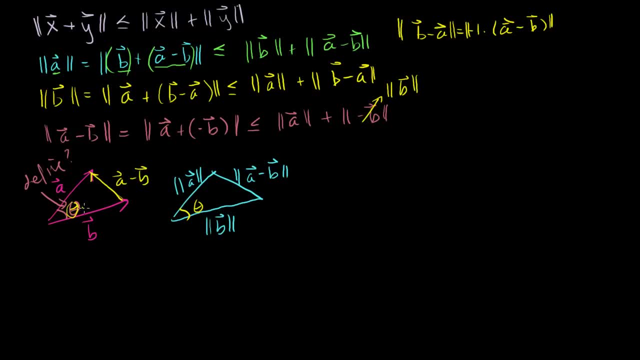 number of components. I'm defining this angle to be the same as this angle, the angle between the two sides, the two lengths of those vectors, in just a regular run-of-the-mill triangle. Now, what can I do with this? 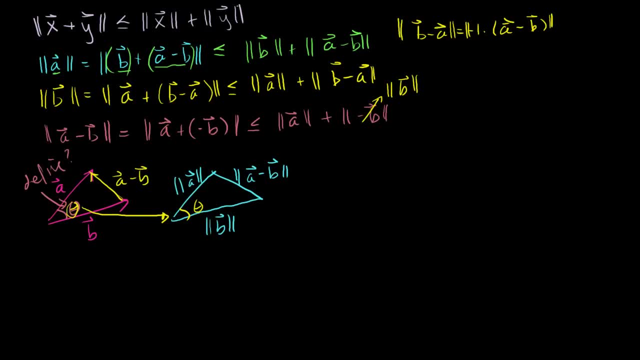 Well, can we find a relationship between all of these things right here? Well, sure, If you remember from your trigonometry class, you have the Law of Cosines, And if you don't, we have a. I've proved it in their. 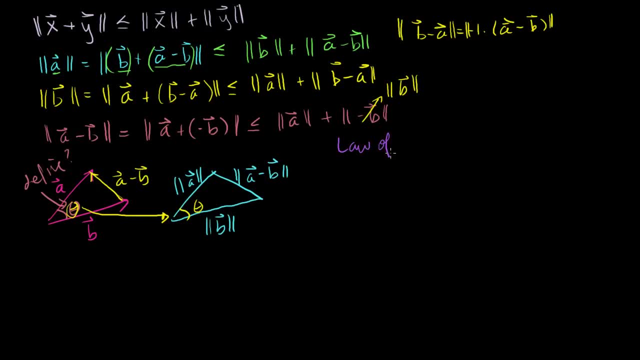 playlist. you have the Law of Cosines And I'll do it with an arbitrary triangle right here, just because I don't want to confuse you. So if this is side A, B and C and this is theta, the Law, 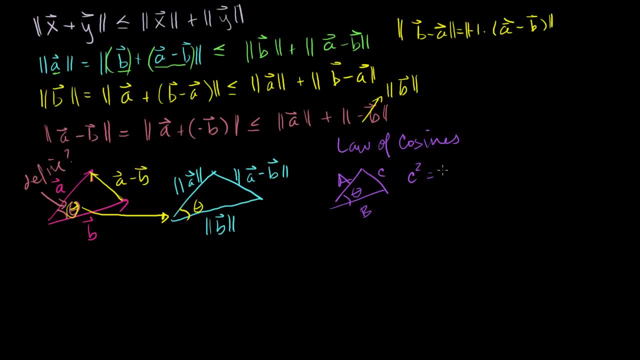 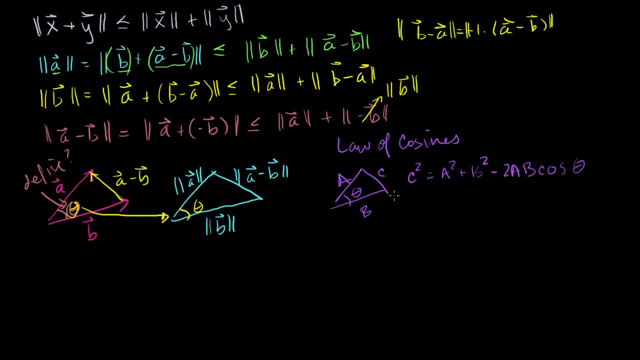 And that's the law of cosines, of theta. I always think of it as kind of a more broader Pythagorean theorem, because this thing does not have to be a right angle, It accounts for all angles. If this becomes a right angle, then this term disappears and 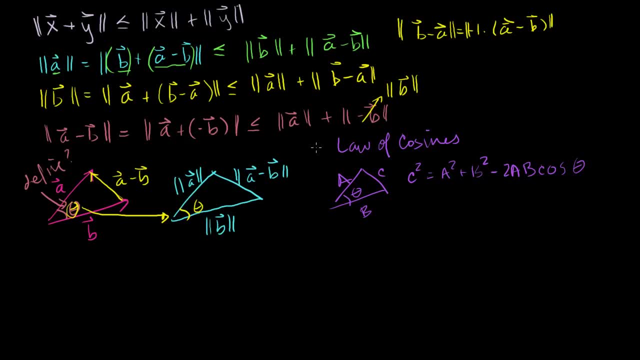 you're just left with the Pythagorean theorem, But we've proven this. This applies to just regular run-of-the-mill triangles- And, lucky for us, we have a regular run-of-the-mill triangle here, So let's apply the law of cosines to this. 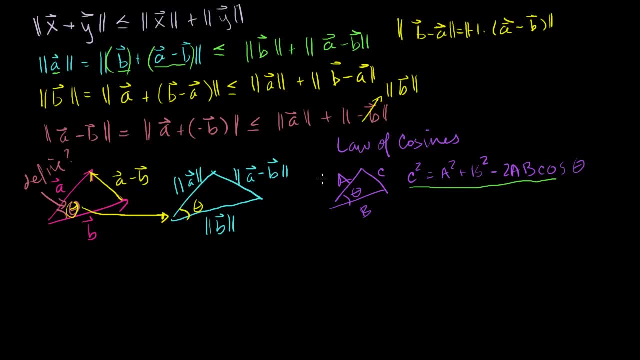 triangle right here. So we would get- and the way I drew it they correspond- The length of this side squared. so that means the length of a minus b squared, The length of vector a minus vector b. that's just the length of that side. 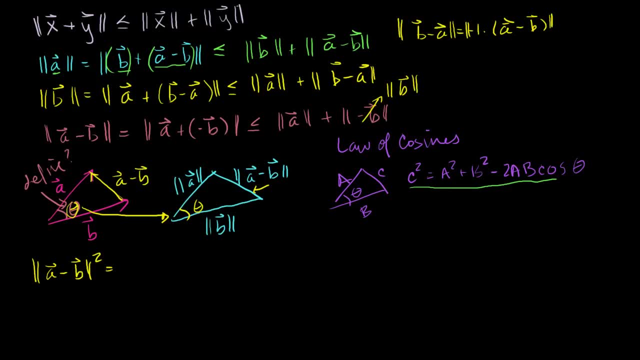 So I'm just squaring that side. It equals the length of vector b squared plus the length of vector a squared Minus 2.. 2 times the length of vector a, times the length of vector b, times the cosine of this angle right here. 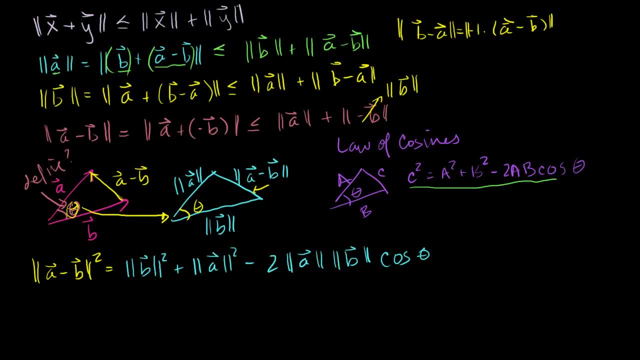 Times the cosine of that angle, And I'm defining this angle between these two vectors to be the same as this angle, right there. So, if we know this angle by definition, we know that angle, right there. Well, we know that the square of our lengths of a vector 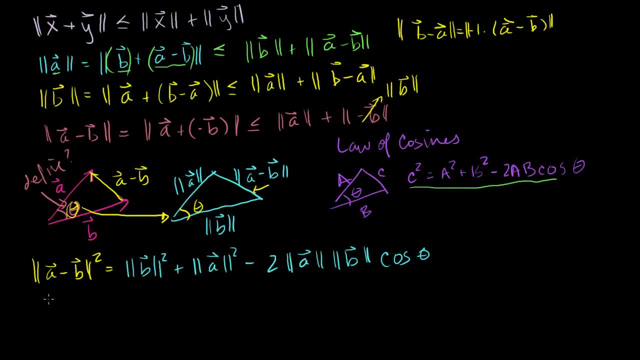 when we use our vector definition of length, that this is just the same thing as a vector dotted with itself. So that's a minus b, dot a minus b, And it's all going to be equal to this whole stuff on the right-hand side. 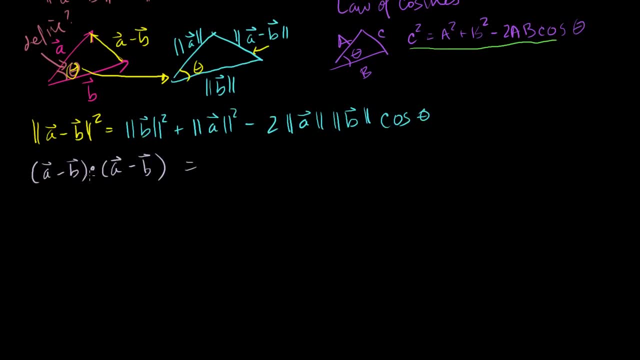 But let me simplify the left-hand side of this equation: a minus b, dot a minus b. This is the same thing as a, dot, a, right, Those two terms Minus a, dot b, Minus a- dot b, And then I have minus b- dot a. 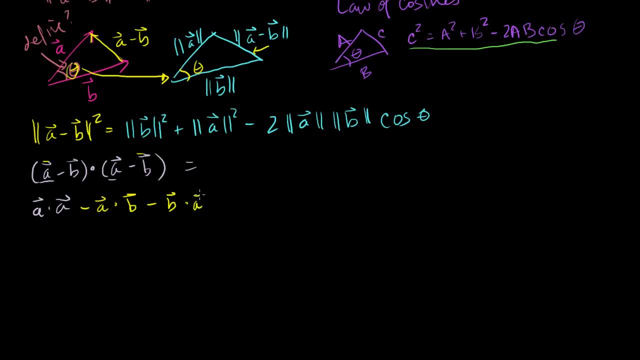 Minus b- dot a. That's those two terms right there. And then you have the minus b- dot minus b. That's the same thing as a plus b- dot b. Remember, this is just a simplification of the left-hand side. 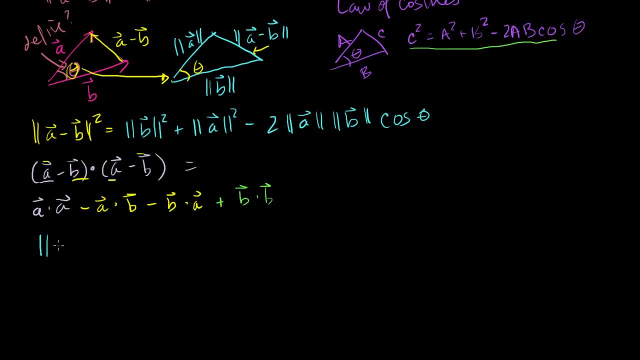 And I can rewrite this: a dot a. we know that's just the length of a squared a dot b and b dot a are the same thing, So we have two of these. So this right here, This term, right there, We'll simplify to minus 2 times: a dot b. 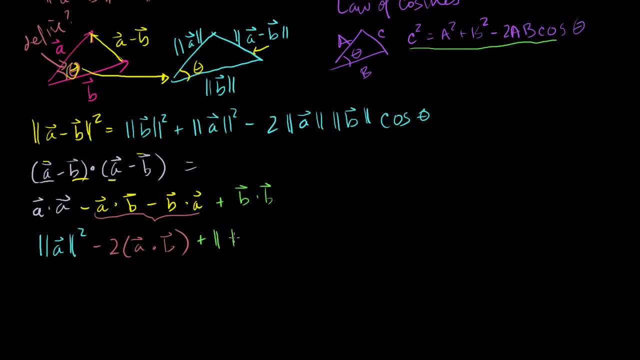 And then finally b dot b. We know that that's just the length of b squared. Now I just simplified, or maybe I just expanded. That's a better word. When you go from one term here to three terms, you can't say: 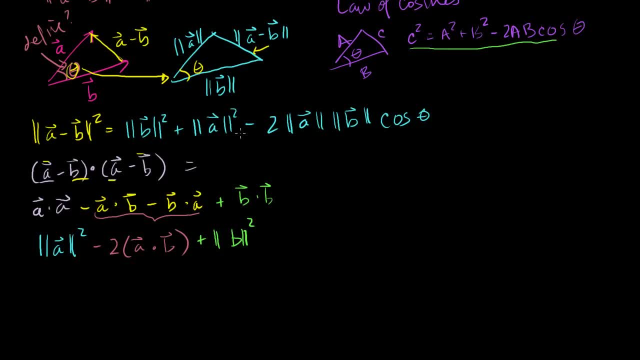 you simplified it, But I expanded just the left-hand side. So this has to be equal to the right-hand side by the law of cosines. So that is equal to. Instead of rewriting it, let me just copy and paste it. What did I just do? 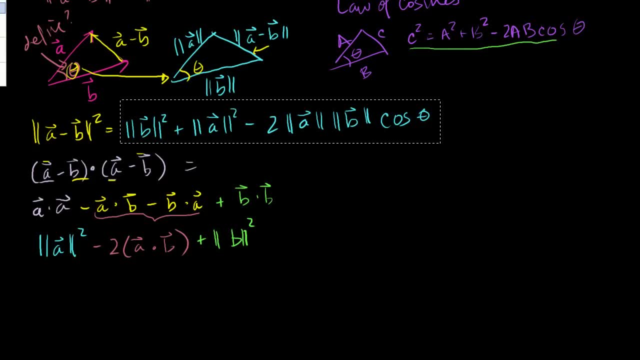 Copy and then edit. Copy and paste. There you go. I don't know if that was worth it, but maybe I saved a little bit of time. So that is equal to that right there, And then we can simplify. We have a length of a squared here. length of a squared. 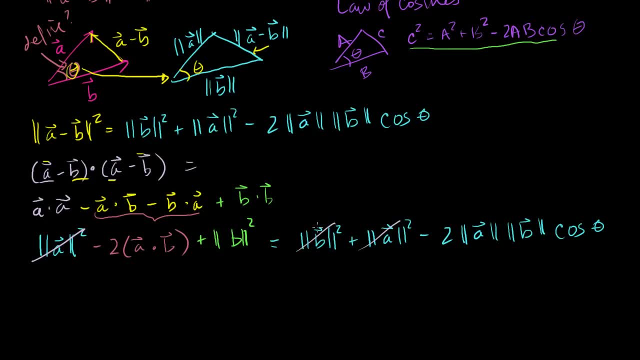 there, Subtract it from both sides. Length of b squared here: length of b squared there, Subtract it from both sides. And then what can we do? We can divide both sides by minus 2, because everything else has disappeared, And so that term and that term will both become ones. 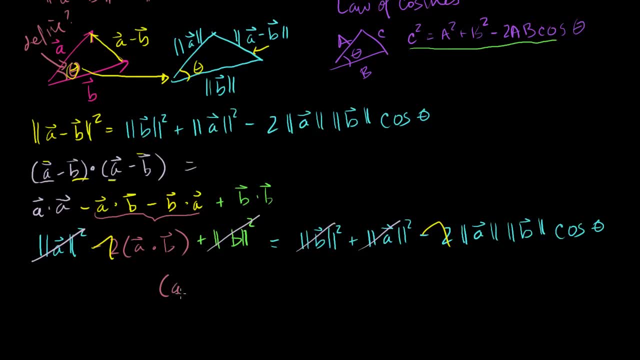 And all we're left with is the vector a dot the vector b. And this is interesting because all of a sudden we're getting a relationship between the dot products of two vectors- We've kind of gone away from their definition by lengths- but that the dot product of two vectors is equal to the 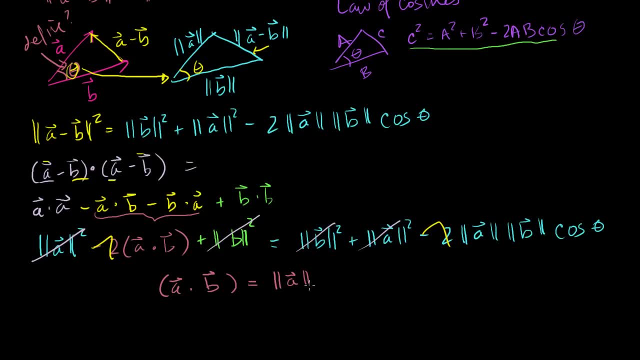 product of their lengths, their vector lengths, and they can have an arbitrary number of components times the cosine of the angle between them. Remember this theta I said this is the same as when you draw this kind of analogous regular triangle, but I'm 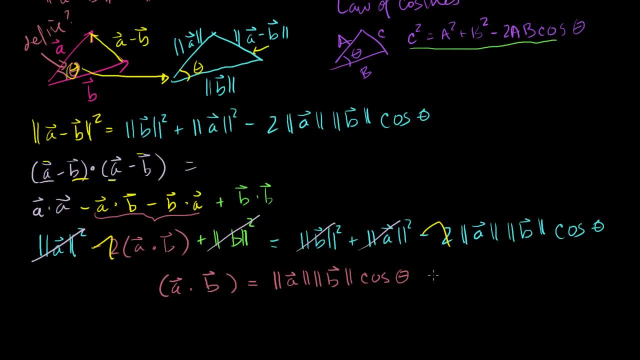 defining the angle. I want the angle between them to be the same as that, So I can say that this is the angle between them And obviously the idea of between two vectors it's hard to visualize if you go beyond three dimensions. but now we 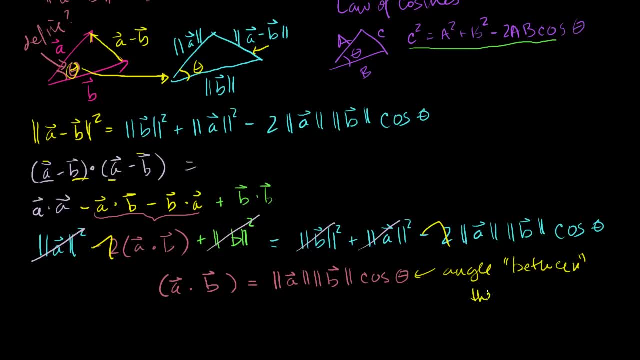 have it at least mathematically defined- Angle between them. So if you give me two vectors, we can now, using this formula that we proved, using this definition up here, we can now then calculate the angle between any two vectors using this right here. 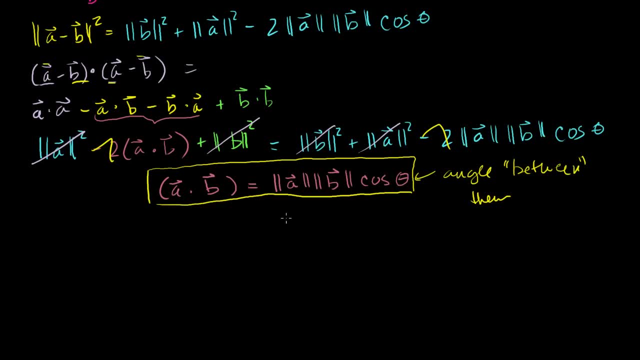 And just to make it clear what happens if a is a, and maybe it's not clear from that definition. so I'll make it clear here that by definition, if a is equal to some scalar multiple of b, where c is greater than 0, we'll define. 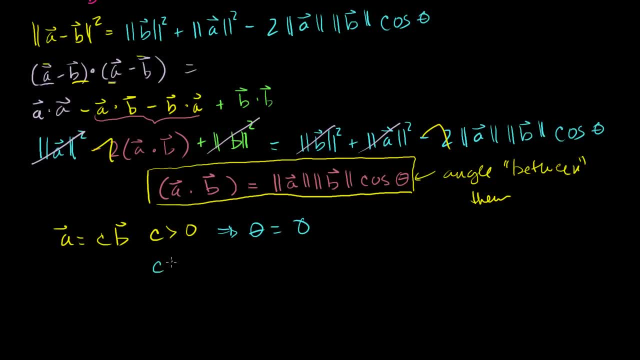 theta to be equal to 0, and if c is less than 0,. so a is a collinear but goes in the exact opposite direction. we'll define theta to be equal to 180 degrees, And that's consistent with what we understand about just. 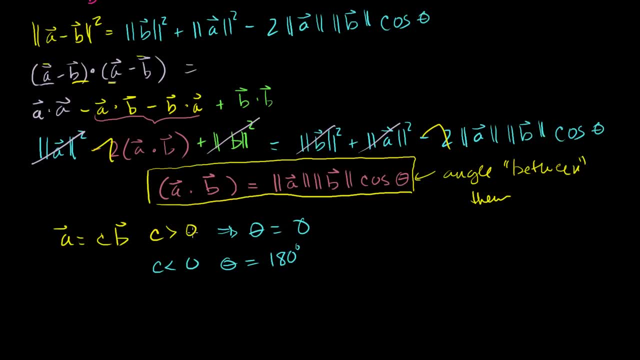 two-dimensional vectors, If they're collinear and kind of the scalar multiple's the same. that means a looks something like that and b looks something like that. So we say, oh, that's a 0 angle. And if they go the other way, if a looks something like 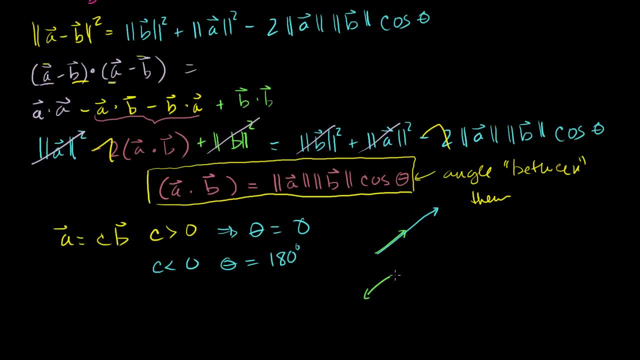 this is the case where a is just going in the other direction from b. a goes like that And b goes like that. We define the angle between them to be 180 degrees, But everything else is pretty well defined by the triangle example. 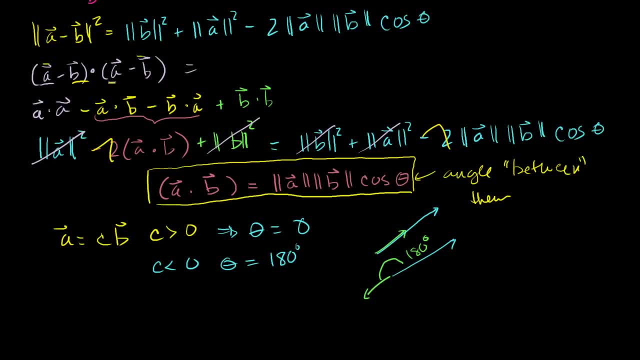 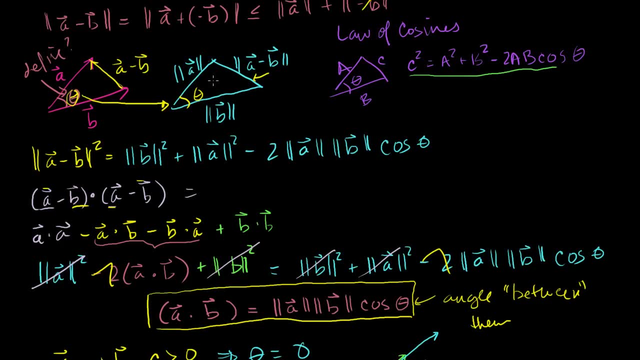 I had to make the special case of these because it's not clear. you really get a triangle in these cases, because then the triangle kind of disappears. It flattens out if a and b are on top of each other or if they're going in the exact opposite direction. 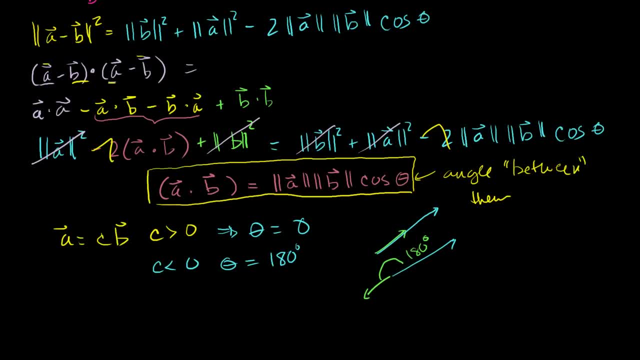 So that's why I wanted to make a little bit of a side note right there. Now We can, Using this definition of the angle between the vectors, we can now define the idea of perpendicular vectors. So we can now say perpendicular vectors, this is: 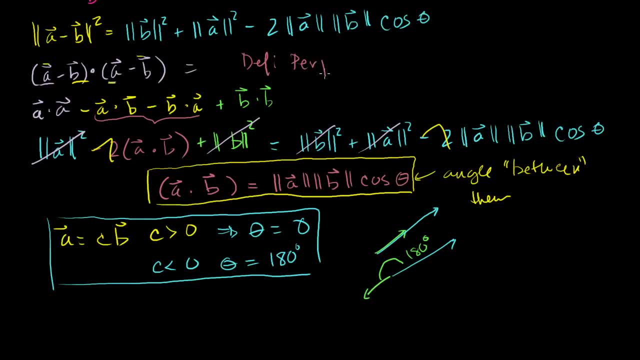 another definition: Perpendicular, And this won't be earth shattering, but it kind of is, because we've generalized this to vectors that have an arbitrary number of components. We're defining perpendicular to mean the theta between. so two vectors, a and b, are perpendicular. 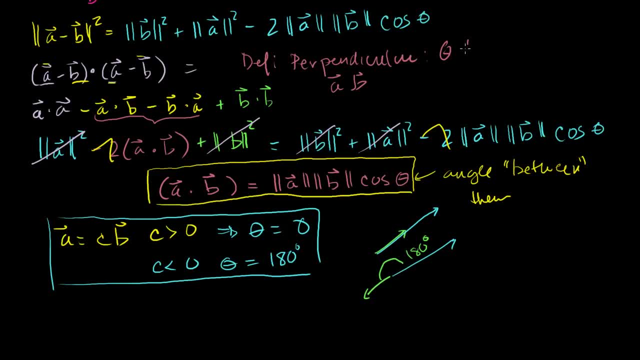 If the angle between them is 90 degrees And we can define that. We can take two vectors, dot them, take their dot product, figure out their two lengths and then you could figure out their angle between them And if it's 90 degrees you can say that they are. 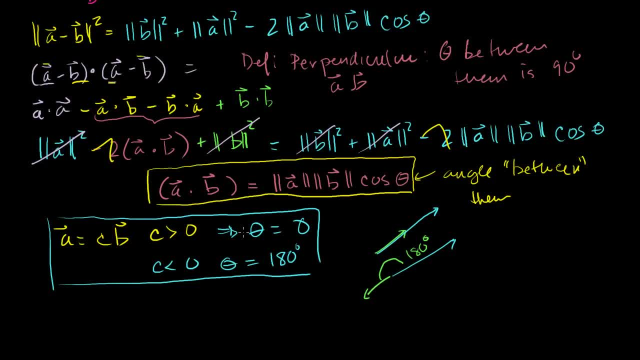 perpendicular angles, And I want to be very clear here that this is actually not defined for this. This is defined for the zero vector, right here. So this situation, this situation right here, not defined for the zero vector, Because if you have the zero vector, then this quantity 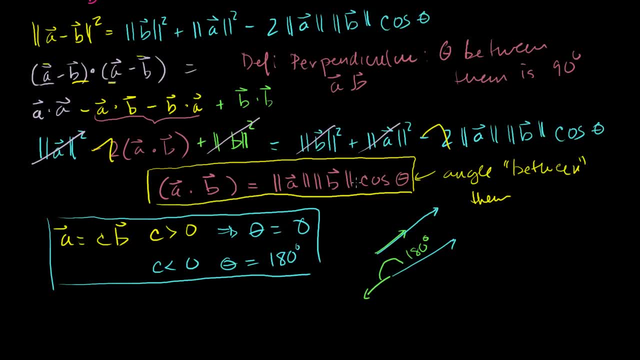 right here, is going to be zero. And then this quantity right here is going to be zero, And there's no clear definition for your angle, right? If this is zero, right here you'd get zero is equal to zero times cosine of theta. 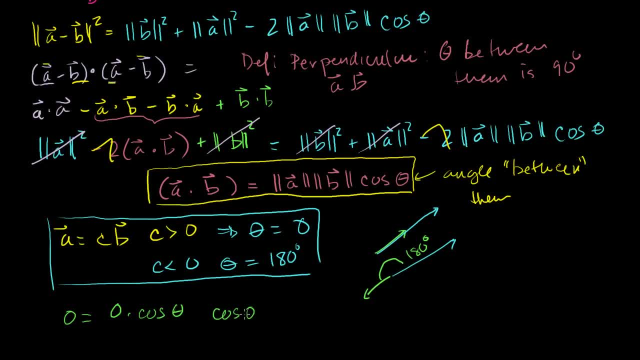 And so if you wanted to solve for theta, you'd get: cosine of theta Is equal to zero over theta, Or zero, which is undefined. But what we can do is create a slightly more general word than the word perpendicular. So the perpendicular you have to have a defined angle to even. 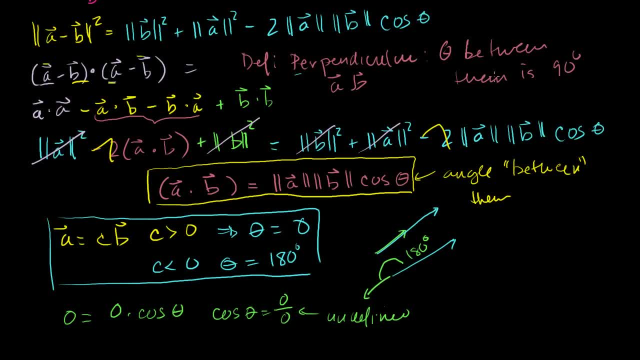 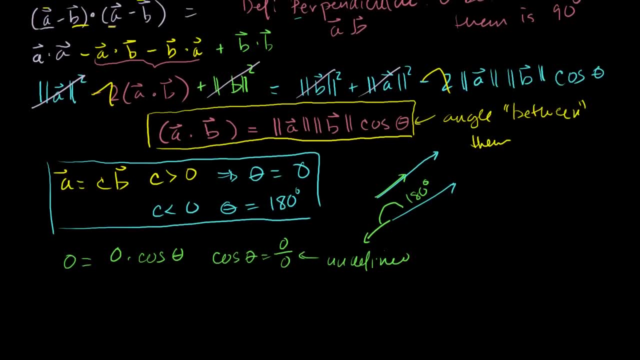 talk about perpendicular. If the angle between two vectors is 90 degrees, we're saying, by definition, those two vectors are perpendicular. But what if we made the statement- and we can, if you look at them, if the angle between two vectors is 90, 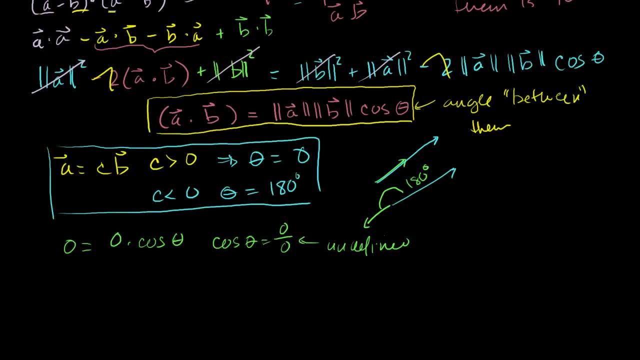 degrees. what does that mean? So let's say that theta is 90 degrees. Let me draw a line here. Let's say that theta is 90 degrees. Theta is equal to 90 degrees. What does this formula tell us? It tells us that a dot b is equal to the length of a times. 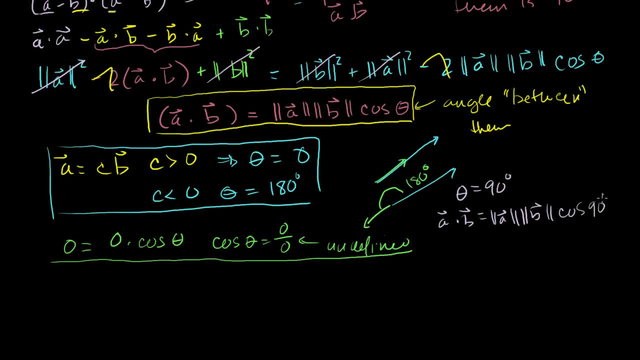 the length of b times cosine of 90 degrees. Well, what's cosine of 90 degrees? It's zero. You can review your unit circle if that doesn't make a lot of sense, But that is equal to zero. So this whole term is going to be equal to zero. 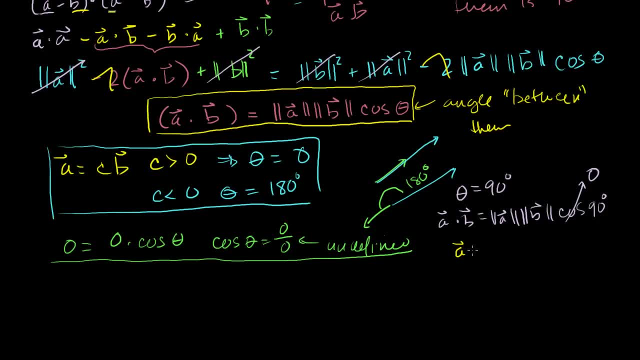 So if theta is equal to 90 degrees, then a dot b is equal to zero. And so- this is another interesting takeaway- If a and b are perpendicular, then their dot product is going to be equal to zero. Now, if their dot product is equal to zero, can we? 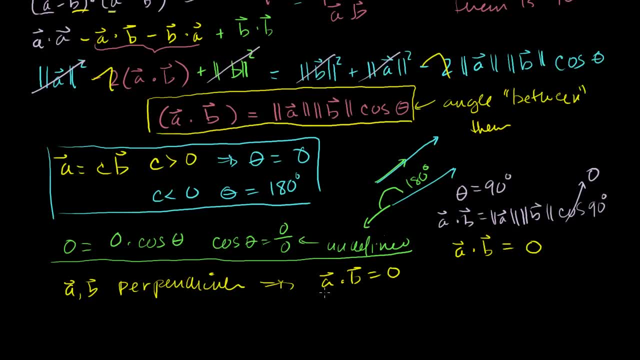 necessarily say that they are perpendicular. Well, what if a or b is the zero vector, The zero vector? let me call z for zero vector, I mean, or I could just draw the. what if the zero vector dot? anything is always going to be equal to zero? 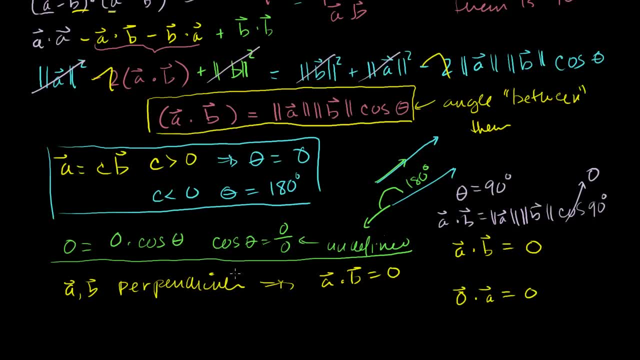 So does that mean that the zero vector is perpendicular to everything? Well, no, Because the zero vector. I said we have to have the notion of an angle between things in order to use the word perpendicular, So we can't use the zero vector. 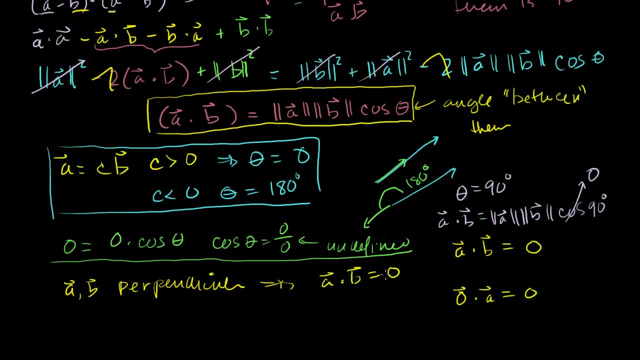 We can't say, just because two vectors dot products are equal to zero, that they are perpendicular, And that's because the zero vector would mess that up, because the zero vector is not defined. But if we say- and we have been saying- that a and b are, 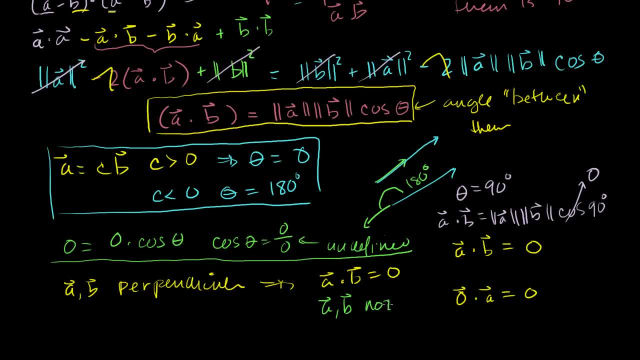 non-zero. if they are non-zero vectors, then we can say that if a and b are non-zero, then we can say that if a and b are non-zero and their dot product is equal to zero, then a and b are perpendicular. 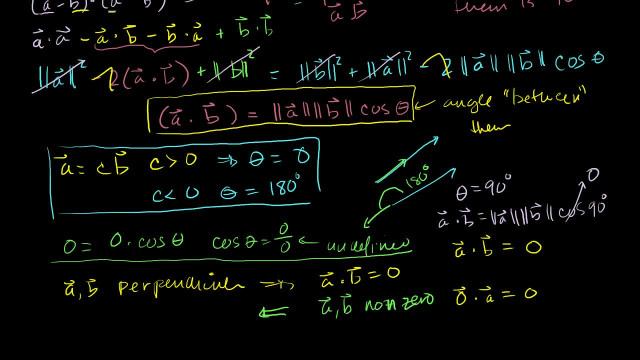 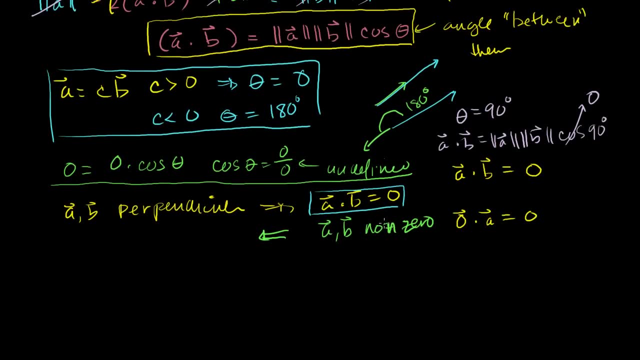 So now it goes both ways. But what if we just have this condition right here? What if we just have the condition that a dot b is equal to zero? It seems like that's kind of just a simple, pure condition And we can write a word for that. 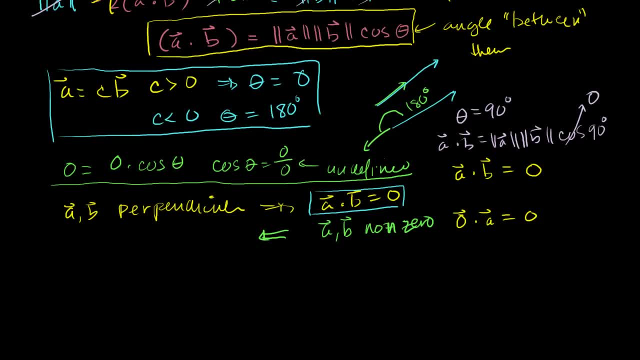 And these words are often used synonymously, but hopefully you understand the distinction. now We can say that if two vectors dot product is equal to zero, we will call them. We'll call them orthogonal, As I always say, spelling isn't my best subject. 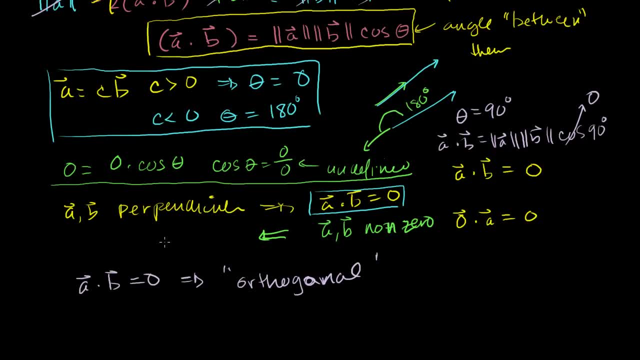 But this is kind of a neat idea. This tells us that all perpendicular vectors are orthogonal, and it also tells us that the zero vector is orthogonal. Orthogonal to everything else, To everything, Even to itself The 0, dot 0 vector, you still get 0. 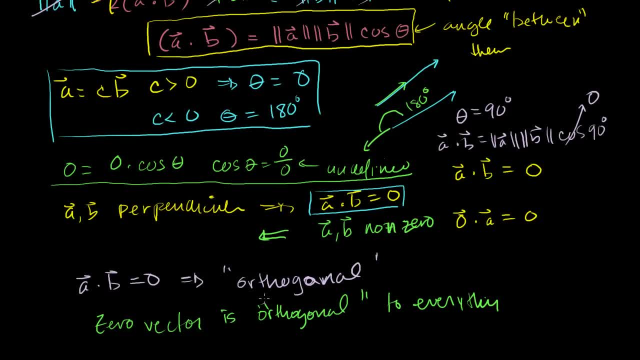 So by definition it's orthogonal. So for the first time probably in your mathematical career, you're seeing that the words- every time you first got exposed to the words perpendicular and orthogonal in geometry or maybe in physics or wherever else, they were always kind of the same words. 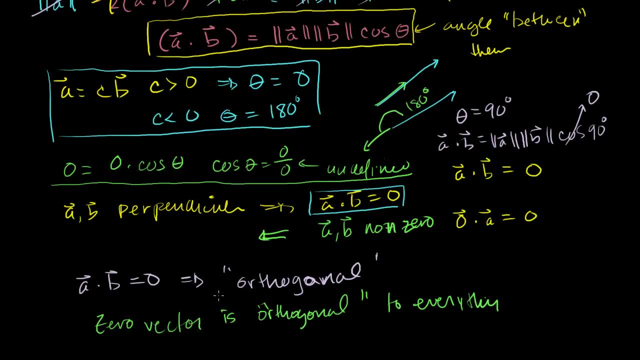 But now I'm introducing a nice little distinction here, and you can kind of you know I'm going to be a little smart aleck with teachers. Oh is it? you know it's perpendicular only if the vectors aren't you know, if neither of them are zero. 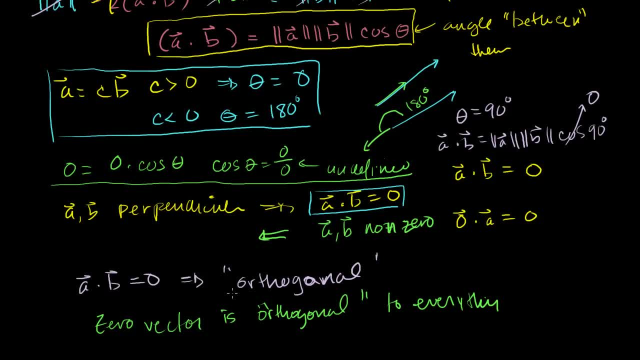 vector. Otherwise, if their dot product is 0, you can only say that they're orthogonal, But if they're non-zero, you could say that they're orthogonal and perpendicular. But anyway, I thought that I would introduce this little distinction for you, in case you have someone who likes to. 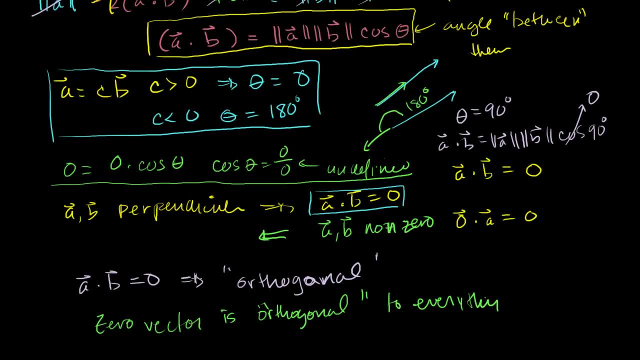 trip you up with words. But it also, I think, highlights that we are building a mathematics from the ground up And we have to be careful about the words we use And we have to be very precise about our definitions, Because if we're not precise about our definitions, then we 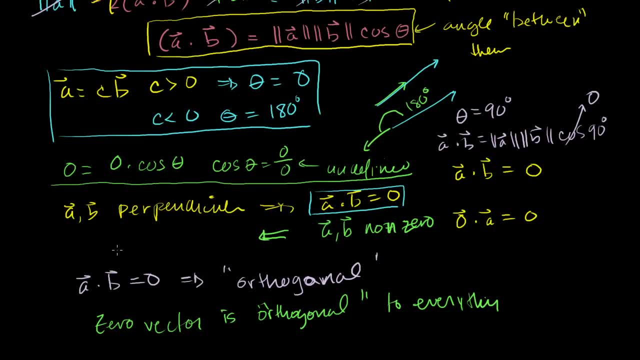 build up a bunch of mathematics on top of this and do a bunch of proofs. one day we might scratch our heads and reach some type of weird ambiguity, And it might have all came out of the fact that we weren't precise enough in defining what some of these terms mean.